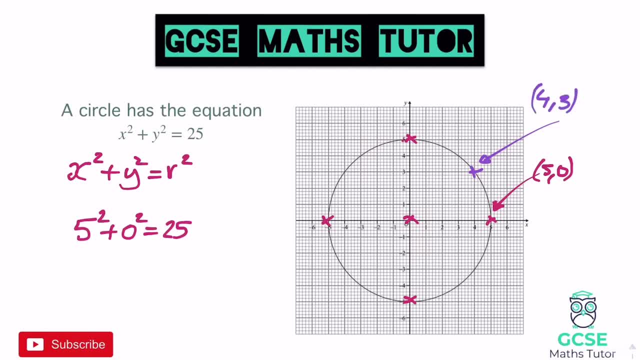 3. And if we sub those points in as well, let's have a look at what we get. We get 4 squared plus 3 squared. 4 squared is 16,, 3 squared is 9, and 16 add 9 is 25.. And that 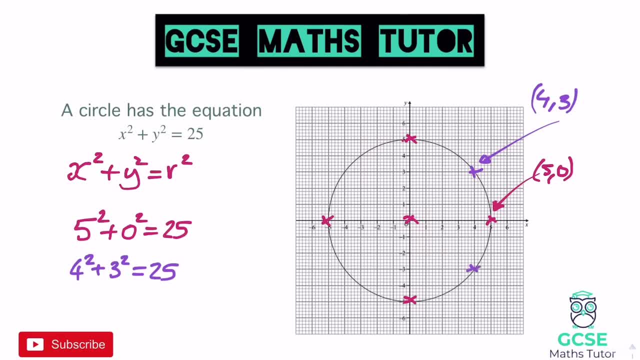 works for all the other 4 3's as well. We've got 4, negative 3,, we've got negative 4, negative 3, and we've got negative 4, positive 3 on this coordinate there And it doesn't matter. 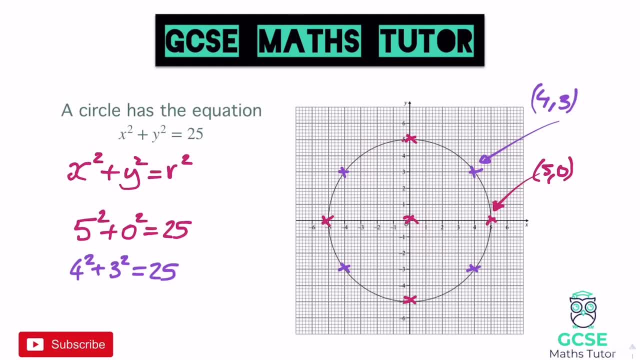 if we sub the negative number in, because negative 4 squared is still 16,. likewise negative 3 squared is still positive 9.. So that gives us those coordinates there And there's a few more that we can actually get. that are whole numbers here. We've got 3, 4 there. 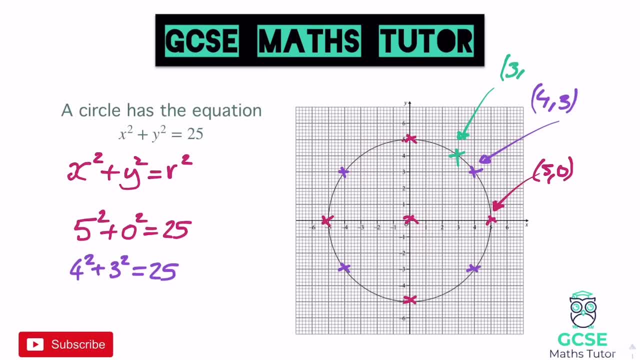 which, again, we can sub in. but it's the same numbers, isn't it? It's just 3 and 4, the other way around, so 3, 4.. And again, you sub those in. obviously we're going to get the same. 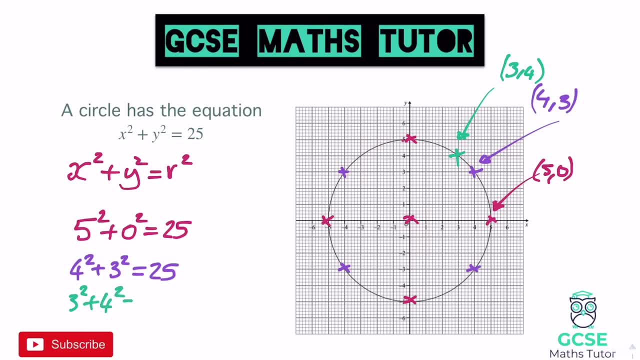 answer here. but 3 squared plus 4 squared is 9 plus 16, which is 25.. These all equal 25.. So you can see why this circle equation actually forms this circle, because you've got the negative 3, 4 there. 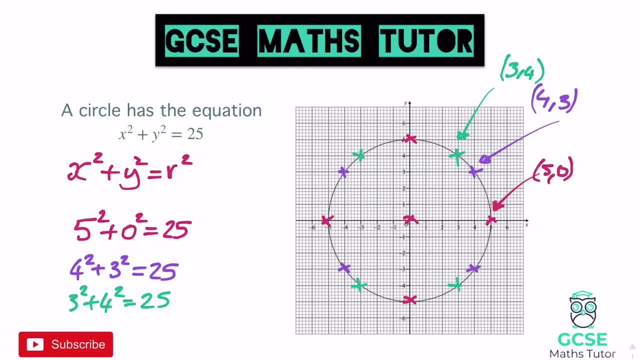 And you've got 3, negative 4 down here. Now they are the only whole number coordinates that work on this circle. But you can kind of see, obviously, how the circle is constructed via this equation now and you can see why it is what it is. But this is what you need. 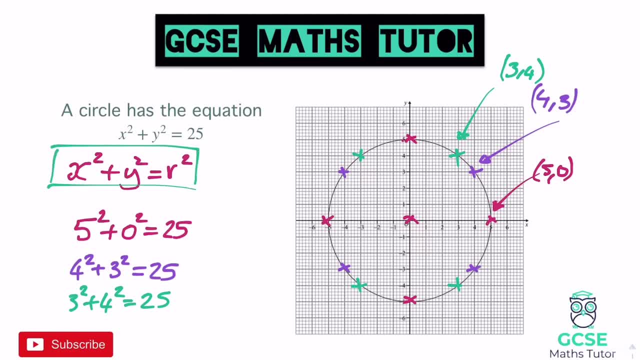 to remember. really, You need to remember: x squared plus y squared equals the radius squared. So, likewise, if we are also trying to find the radius of the circle and we have the equation but no diagram, we would know that, in order to get the radius from the 25, we 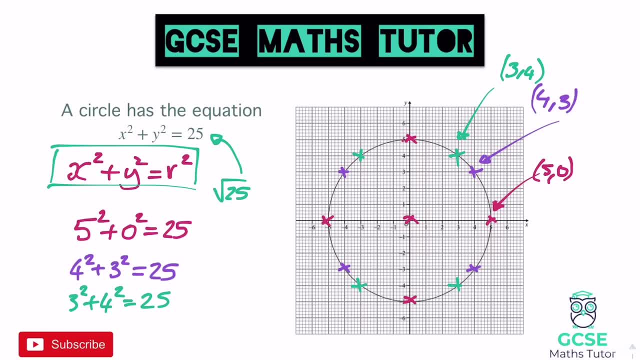 would just do the square root of 25.. That would give us our radius there, which is 5.. And you can see on the diagram: there the radius is 5.. This is very specific to circles with centre 0, 0, though, or at the. 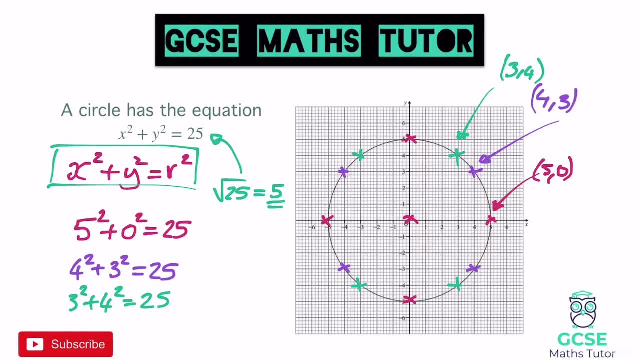 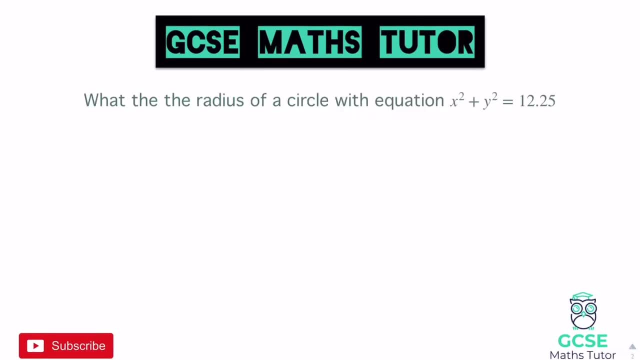 origin, And that's what we're going to be having a look at. obviously, unless it explicitly says that the centre is somewhere else. But let's have a look at a couple of little questions, OK, so a nice quick one here. it says: what is the radius of a circle, with the equation: 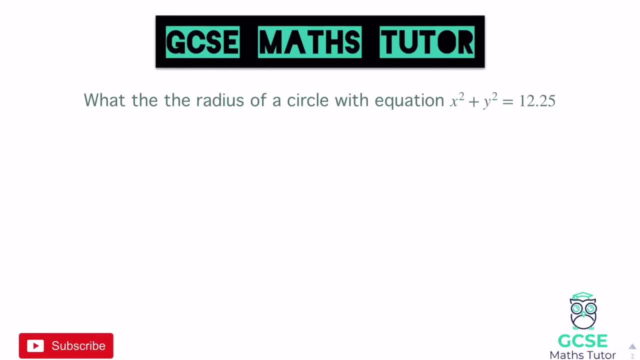 x squared plus y squared equals 12.25?. Obviously it would be a lot easier if the number at the end there was like a nice square number, because obviously it's nice and easy to square root that. So the radius from here we just have the square root, 12.25.. So the square root of 12.25,. 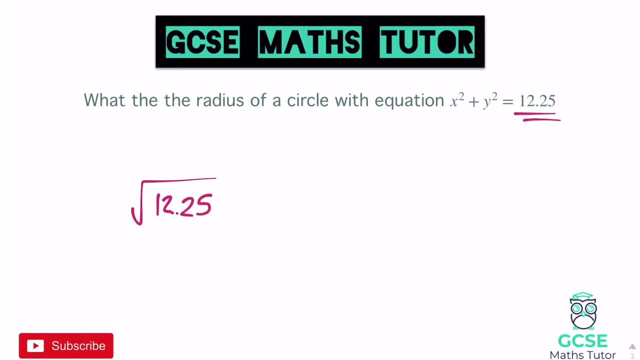 obviously this would be a calculator question? Potentially not. we'll have a look at how to approach it if it wasn't calculator. But if we're on the calculator, the square root of 12.25, and it comes out as 7 over 2, which, if I turn into a decimal, comes out as 3.5.. 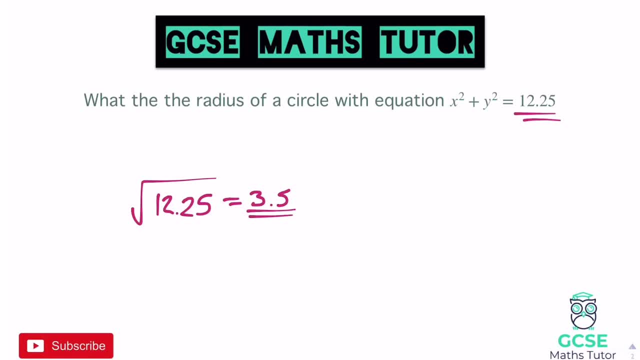 So there's the radius there. Nice and easy with a calculator. If you didn't have a calculator for this, you would have to take a slightly different approach. We'd have to turn that into a fraction, Which would be 12.25.. Make that top heavy. So 12 times the 4 is 48, plus the 1 is 49. So 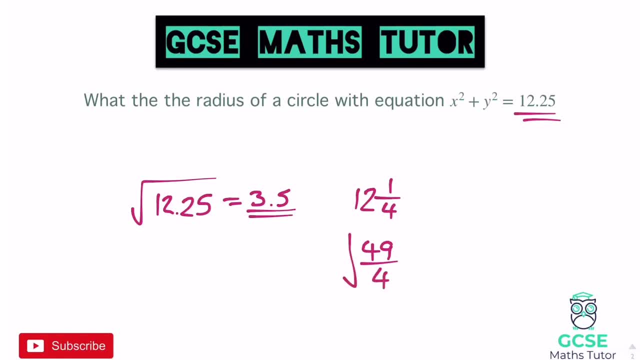 we get 49 over 4.. And then we could square root that, And when you square root that, you can see you've got a nice square number on the top and the bottom there. The square root of 49 is 7.. The square root of 4 is 2.. And we get the answer there: 7 over 2.. Which you 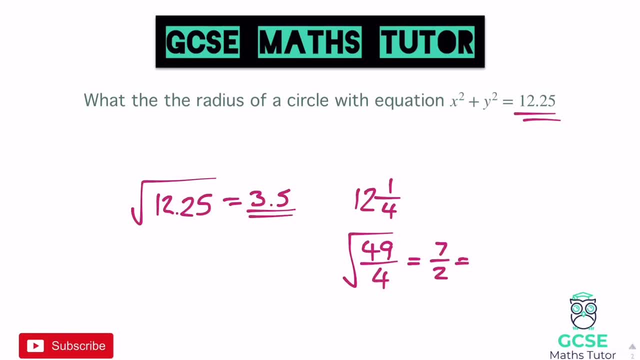 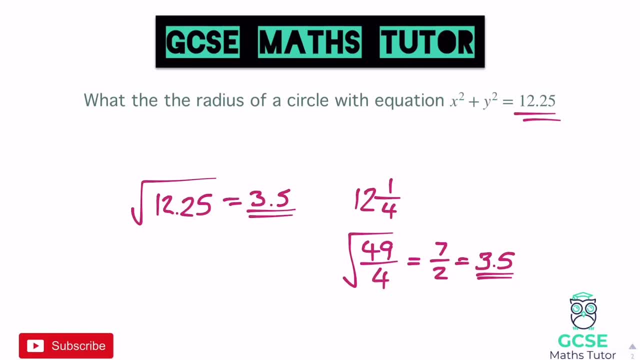 So we can take a little bit of approach there, thinking about how we could do that using non-calculator methods as well. But the majority of the time that is going to be a calculator style question there. Let's have a look at a slightly different question. 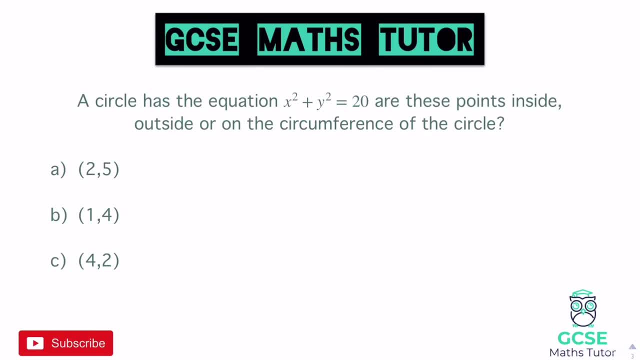 Okay, so a circle has the equation: x squared plus y squared equals 20.. And are these points outside, inside, outside or on the circumference of the circle? Now, we know on the circumference of the circle if these points equal 20.. Because it says that it equals 20 there. So if we 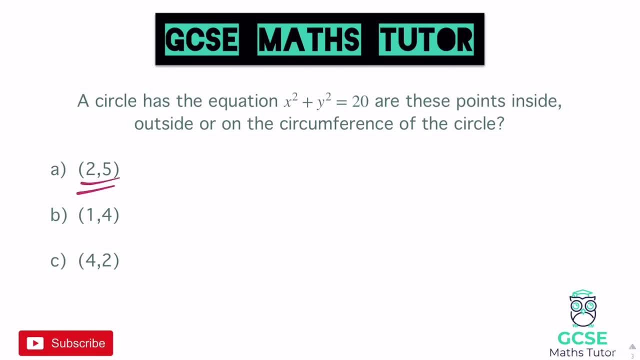 sub them in, let's see what we get. So the first one: 2, 5.. If I sub them in, 2 is the x coordinate there. So 2 squared plus 5 squared, And let's see what we get: 2 squared is 4.. 5 squared is 25.. 4 plus 25. 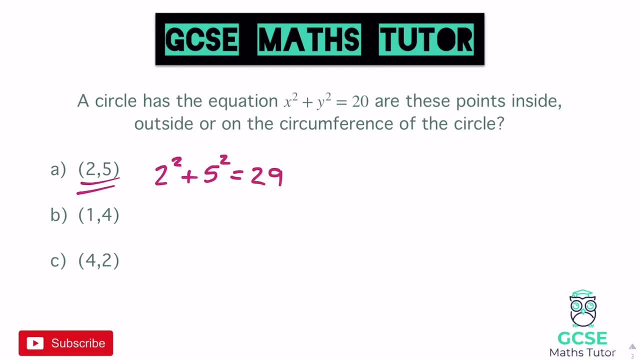 is 29.. So those numbers there are bigger than 20.. And therefore it would be on the outside of the circle. If it's bigger than 20, there 29 is quite a bit bigger, So that would be on the outside of the circle. 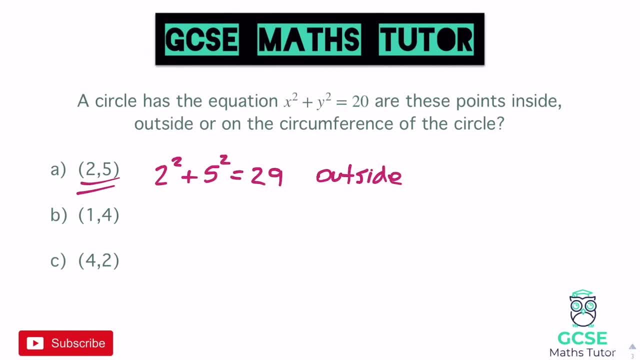 Definitely not on the circumference, which is what we're going to be using this mostly for Looking at if it's on the outside of the circle, If it's on the outside of the circle, If it's on the circumference or not. Let's look at this next one. So, subbing those in The x coordinate, there is 1.. So 1 squared. 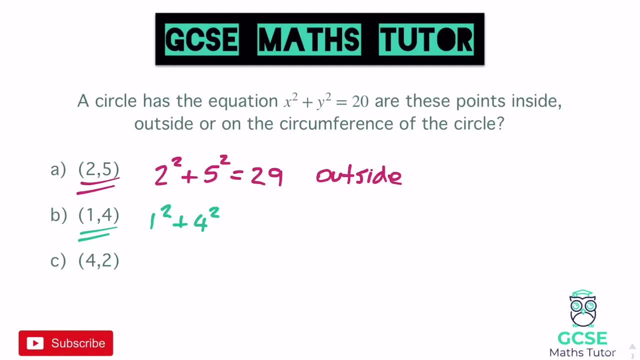 4 squared. What does that equal? 1 plus 16.. 1 plus 16 is 17. That's less than 20.. So that's on the inside of the circle. There we go. Those coordinates are not big enough to equal. 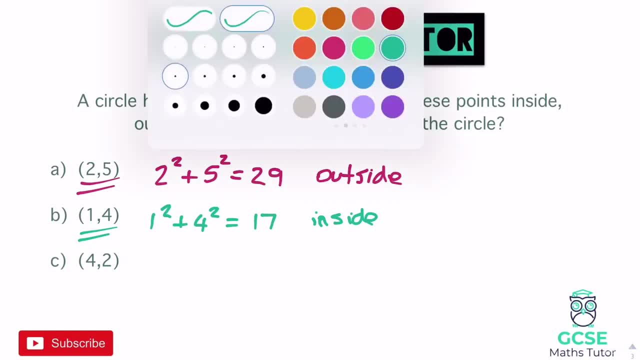 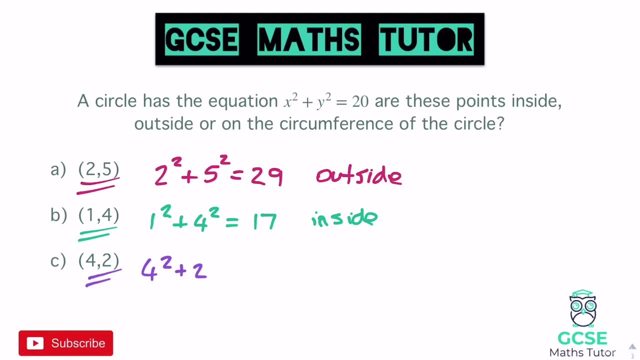 that 20. there. that dictates whether it's on the circumference. And then, moving on to the last one, 4 and 2. If we sub those in, we get 4 squared 4 Add 2 squared. 4 squared is 16, 2 squared is 4, and 16 plus 4 equals 20.. There we go. 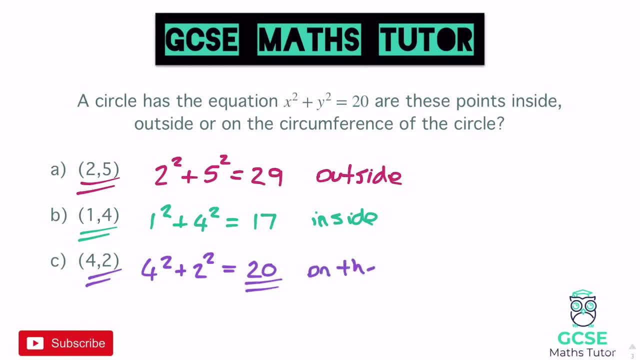 So that would be on the circumference. There we go, and this is really just going to be used just to be aware of the fact that if we have a point on the circumference, it definitely fits within that equation there, and that can be quite handy if we only know one of the coordinates. So take, for example, this one: 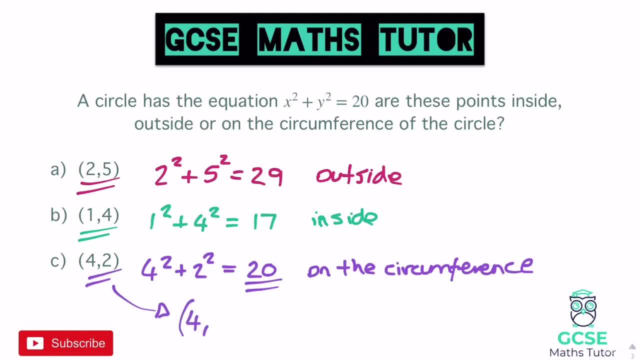 if we only knew that the coordinate was 4, something- let's call that something- x, we could find out what that coordinate is, because we know it has to equal 20 and we could sub it in that we'd get 4 squared plus x squared, equaling 20.. We 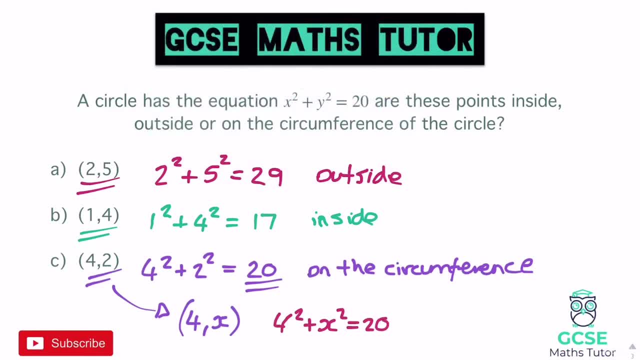 could just solve that like an equation: 4 squared is 16, so we could take away 16 from both sides and we get x squared equals 4, and then we could square root that and get x equals 2, and there's our coordinate 2 that we knew it was. 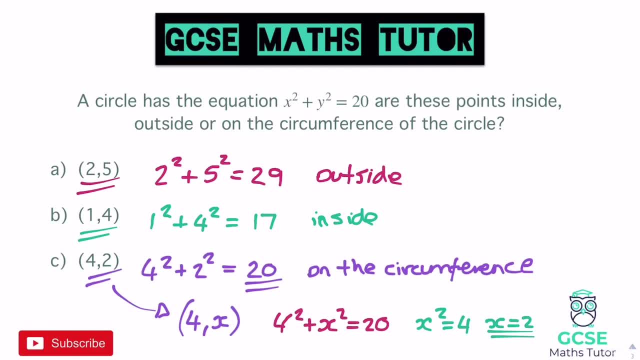 anyway. But we can take that approach, obviously, knowing that they have to equal 20 or whatever the equation of the circle is, we can take that approach to know that it has to balance and therefore we can find any missing coordinates as well, And obviously just having that little bit of an understanding if the number's 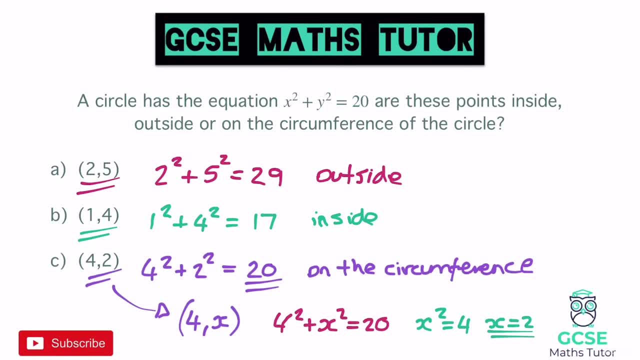 bigger it's outside and if it's smaller it's on the inside. A couple of little questions to practice here. just remember, obviously square root the number at the end to get the radius. We didn't have to in this question. in this case it. 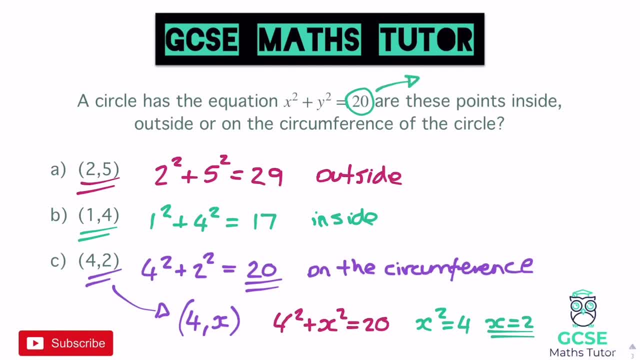 would have given us a third. look, We'd have to do the square root of 20 for the radius, which would give us a third. Obviously, we could look at simplifying that. We're not actually looking at that in this question, but we could simplify that. 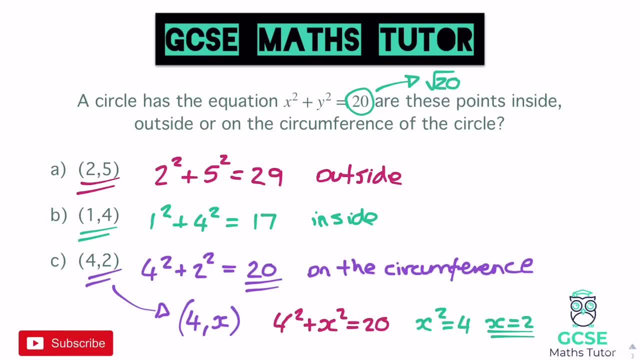 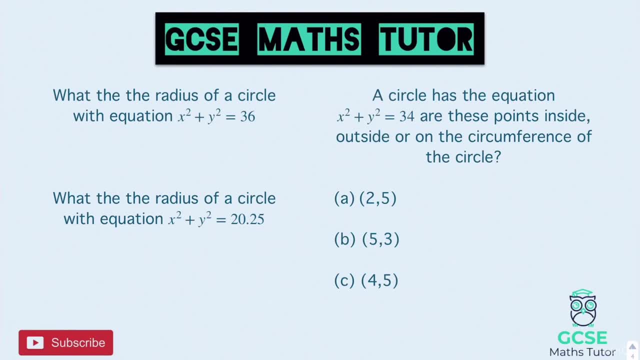 third, but that would be how we would find the radius of this circle as well. So there's a few questions for you to have a go at. Okay, so a few little questions, have a go at these. pause the video there and we'll go over them in a second. Okay, so for the 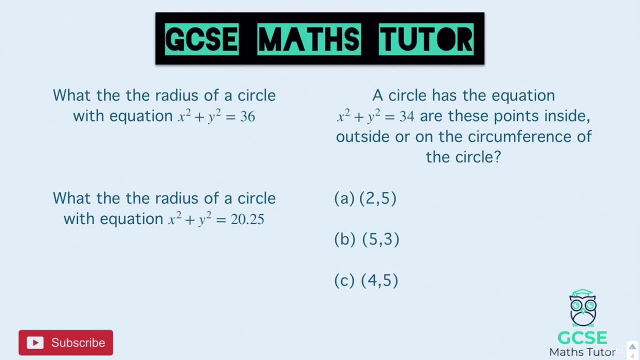 first one radius of this circle. well, we just have to square root that number at the end. So the square root of 36, and that gives us a whole number. nice one there. 6 is our radius. For the next one, we have to do the square root of 20.25.. 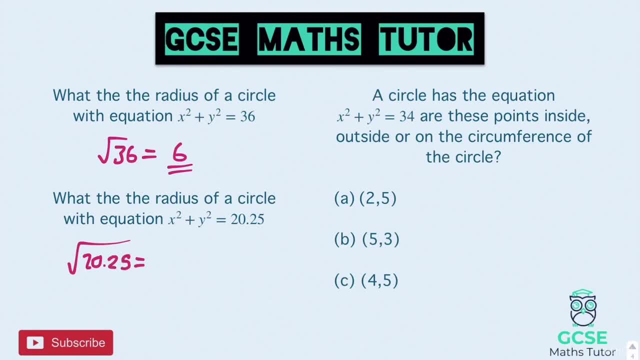 So typing it on the calculator, you get 4.5.. Of course you could have tried doing that without a calculator as well. 20.25 is 20 and a quarter, and if you make that top heavy 20 times 4 is 80 plus the 1 is 81. So it's 81 over 4, and if you square root 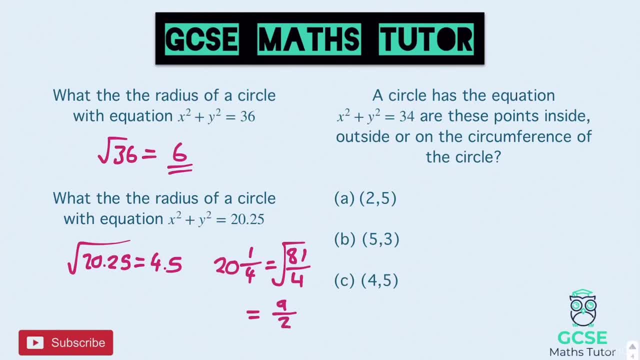 that you get 9 over 2, which is 4.5 as well. So you can use either of those answers and methods of doing it. but there you go. there's a way of doing it without a calculator as well. Right, the last one here. it says a circle has the equation x squared plus y. 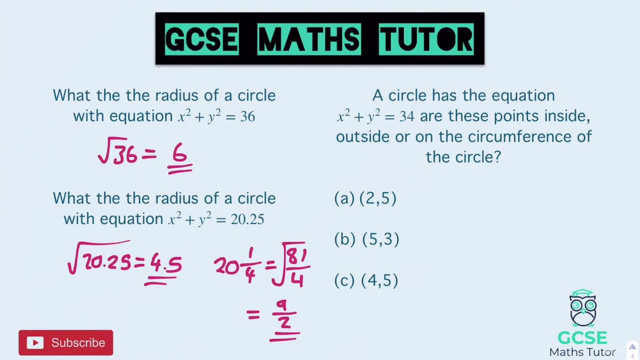 squared equals 34.. Are these inside, outside or on the circumference? So if we sub them in, 2 squared plus 5 squared is 4 plus 25 is 29.. That is smaller than 34, so that's inside. Onto the next one, 5 squared plus 3 squared, which is 25 plus 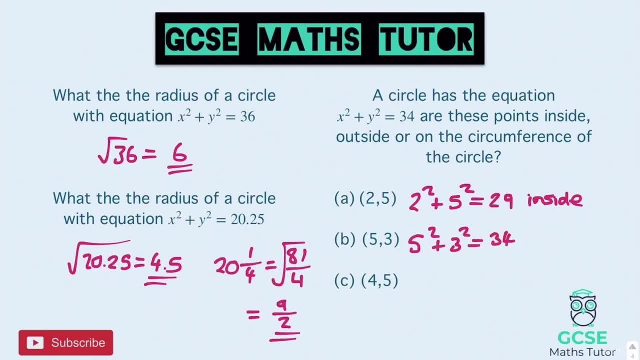 9.. 25 plus 9 is 34.. That's on the circumference. And the last one here: 4 squared plus 5 squared is 16 plus 25, which is 41, which is outside. There you go, bigger than 34 there. Right, there we go. so there's. 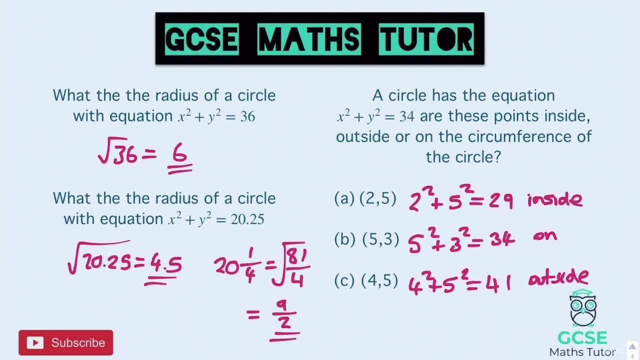 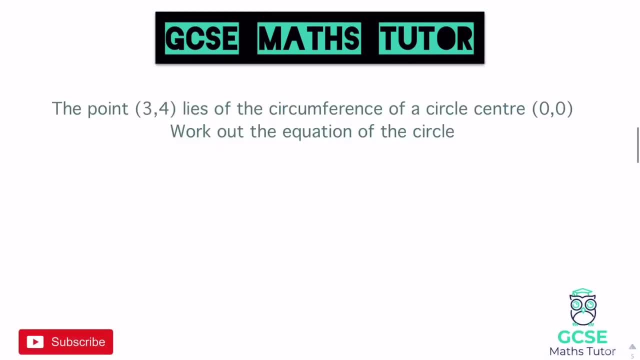 just a bit of an understanding about the actual circle equation, how we can use it to find the radius and also how we can use it to determine if points are on the circumference or not. Let's have a look at actually using this then. Okay, so the 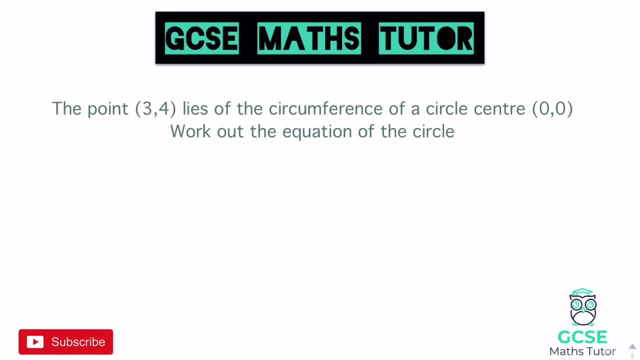 point 34 lies on the circumference of a circle, center 00, work out the equation of the circle. That's quite a nice, actual, easy way of doing this, because if we know that this point is definitely on the circumference, then we can just use. 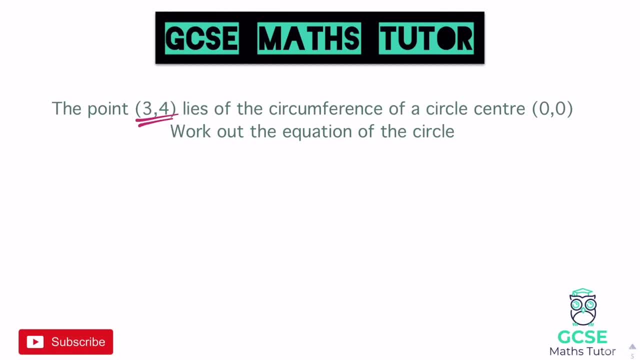 our equation of a circle, and in two different ways I'm going to look at this, but I'm going to start off with this one, because this one is quite a nice one. Now we know the equation of the circle is: x squared plus y squared equals the 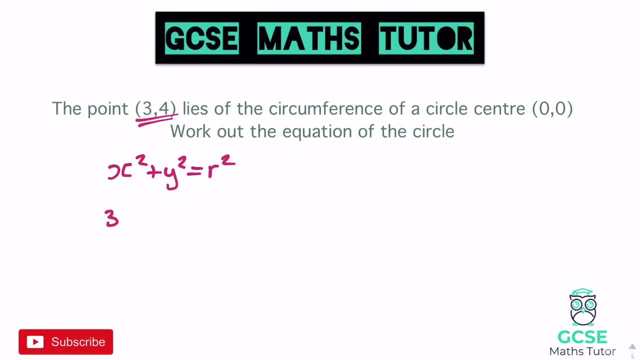 radius squared. So if we just plug these numbers in three, squared being the x coordinate, y being the four, so four squared, and that's going to get us two 9 squared plus 8 squared become 4 squared. So this And that's going to again equal the radius squared. 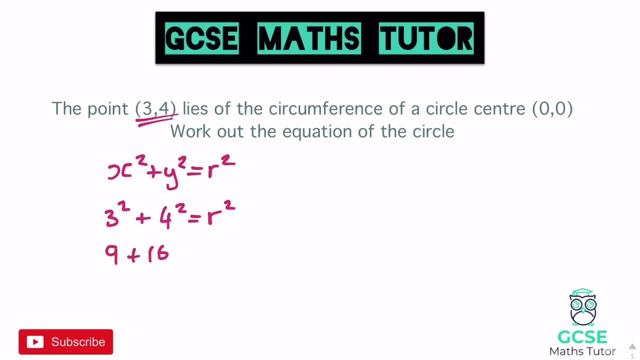 So if we work this out, we'll get 9 plus 16, which equals 25.. Again, that equals the radius squared. So if that equals 25, then we can write our equation there. So we have x squared plus y squared equals 25.. 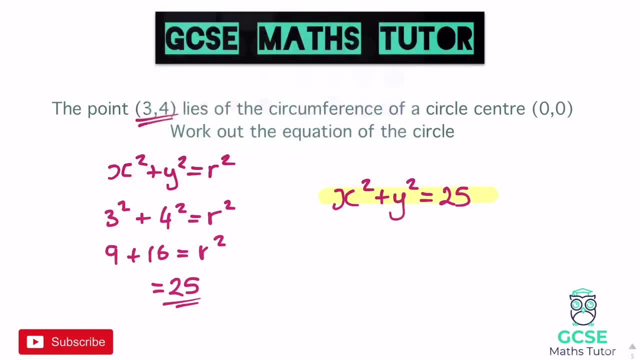 There we go, And although it doesn't ask for it again, we could think about what the radius is here. If we did the square root of 25, we would get 5 as our radius. So obviously that's not part of the question here. 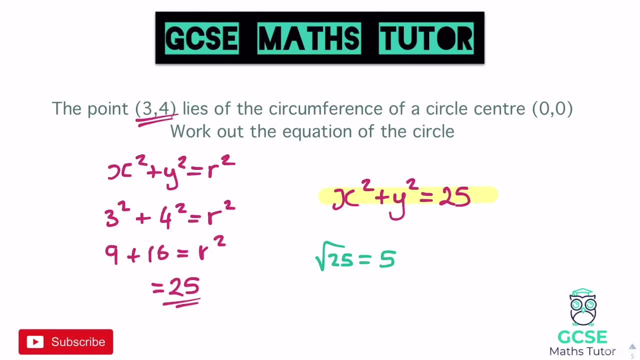 It says: work out the equation of the circle. But just thinking about that as well, you could actually get the radius there as 5.. Now if the centre wasn't at 0, it'd be a little bit trickier to do because we couldn't just sub it straight in. 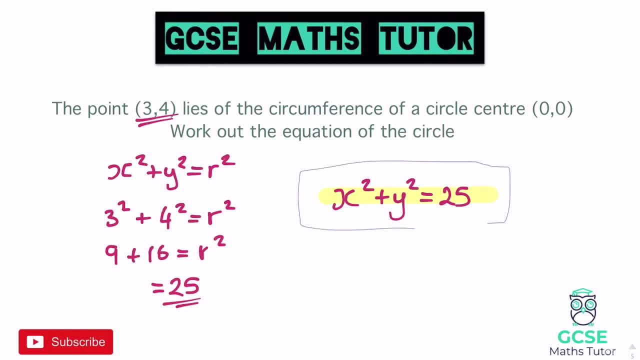 So we'll have a look at another way that you could look at this, because we're going to have a look at one where the equation of the circle there we go is not at centre 0, 0. But if we think about this as a little diagram, 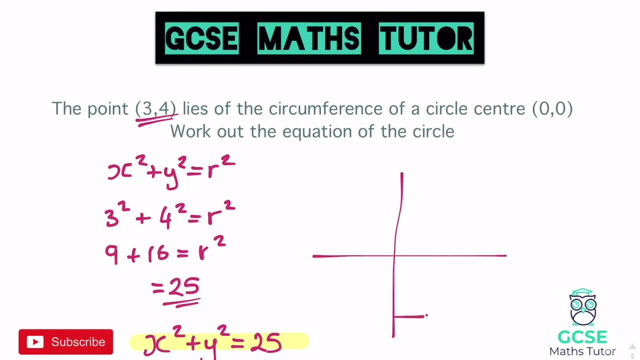 I'm going to go ahead and do that. I'm going to do a little sketch of this. So if we had our circle, we've got centre 0, 0,, 3,, 4.. Let's just say it's up here. 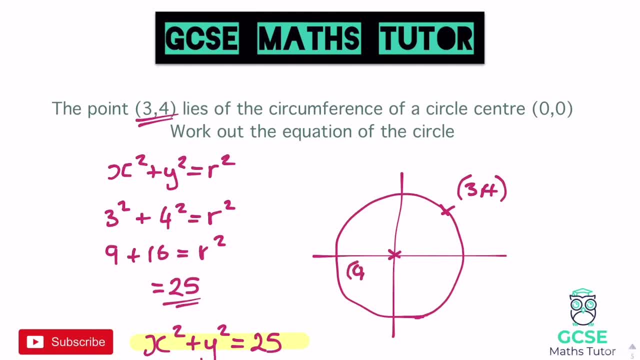 If we wanted to find the length of the radius, which obviously would help us to find the equation of the circle, we could actually draw this in. This is quite a good skill to be able to have here, to be able to do this for the progression of this topic. 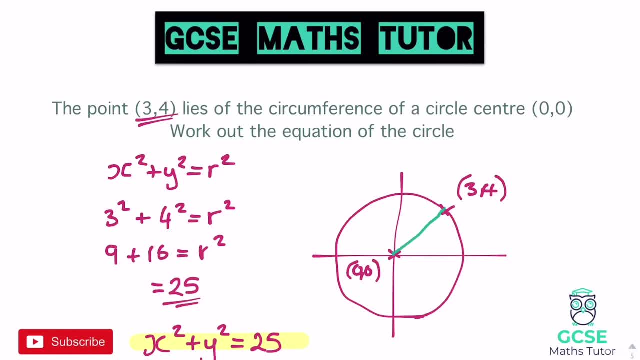 But if we actually draw a line going from 0, 0 to 3, 4 and think about the kind of shape we've got we could make here- So we could make a little right-angled triangle- And thinking about what this little right-angled triangle looks like, 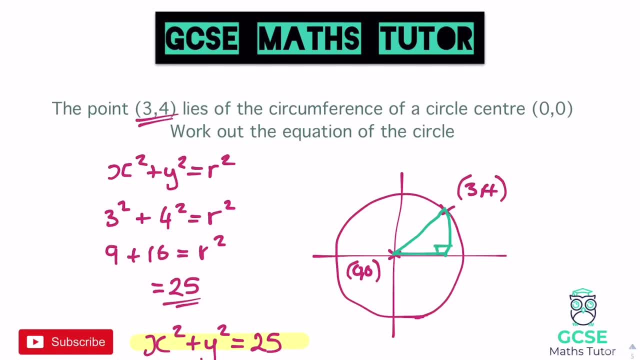 going from 0, 0 to 3, 4,. well, if it goes from 0 to 3 on the x-coordinate, that is, a run here or a change in x of 3, and going from 0 to 4,. 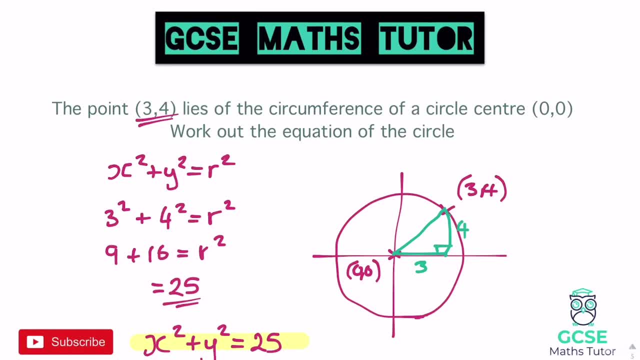 that is a rise or a change in y of 4.. So actually we could use Pythagoras to work out the length of the radius here. So I could just do a bit of Pythagoras. So square them both, add them together and square root them. 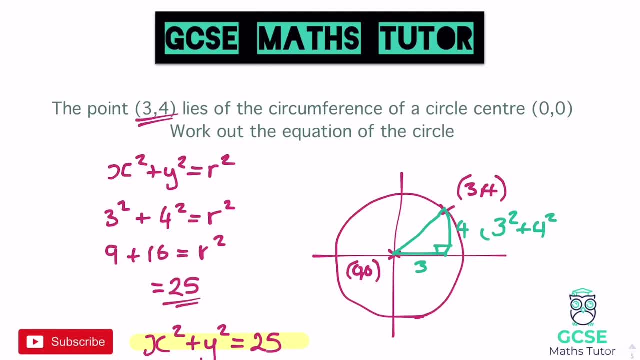 So 3 squared plus 4 squared, And then square root, our answer, which is the square root of 25.. And the square root of 25 is 5.. So there we go. That's another way of showing that the radius is 5.. 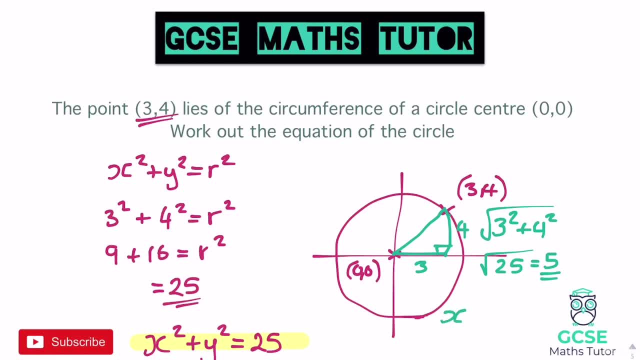 And then, once you've got that, you can obviously put it into your circle equation: x squared plus y squared equals 5 squared, And again squaring that 5 to get you 25, to get your equation of the circle there. 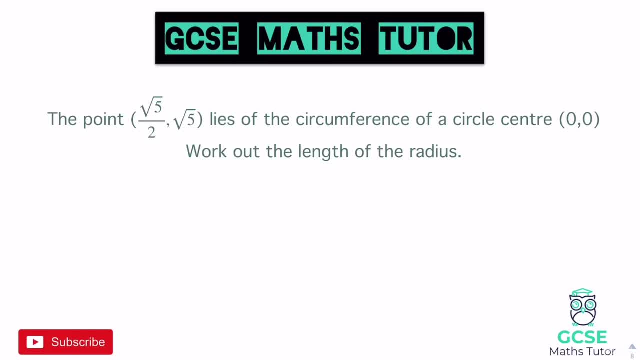 Okay, something slightly tricky here. We've got some thirds involved in the point that's on the circle. So it says this point here: root 5, 5 over 2, and root 5 lies on the circumference of the circle centre 0, 0.. 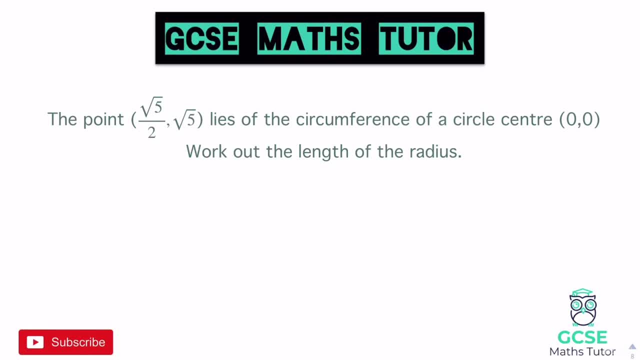 Work out the length of the radius. Okay, so we'll have a look at both here. We'll get the length of the radius and we'll get the equation of the circle as well. But let's just have a look. Now we know we have x squared plus y squared equals r squared. 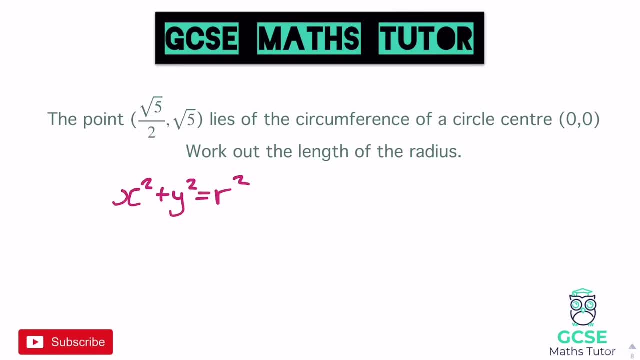 There we go. It's at centre 0, 0.. So we can just sub this point straight in. So if we sub them in our x coordinate, there would be root 5 over 2 squared Plus root 5 squared. 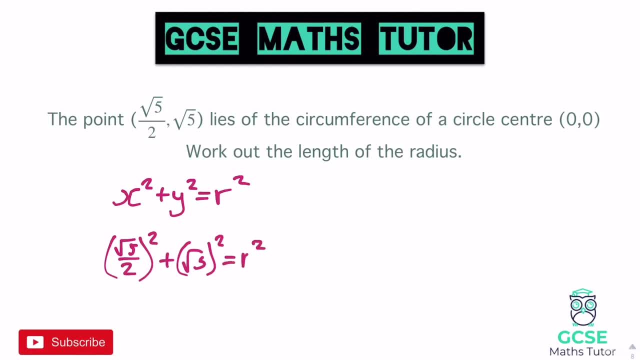 And that's going to equal r squared. And obviously, if you're not sure about thirds here, it would be wise just to have a look at my thirds video, which is in my playlists in the number section or in the thirds section. You can have a little look at some of the thirds there. 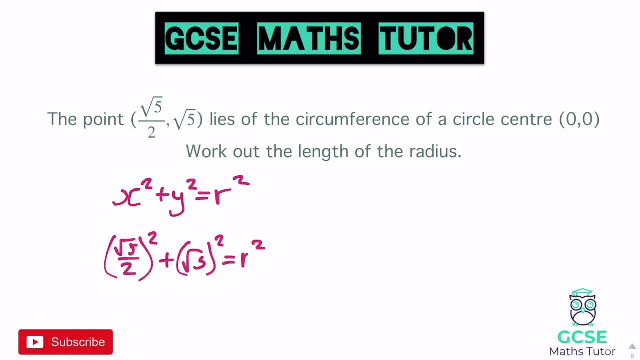 But just thinking about how we treat thirds. So root 5 over 2.. So if we square the top root 5 times root 5 on the top is just 5.. And 2 times 2 on the bottom is 4.. 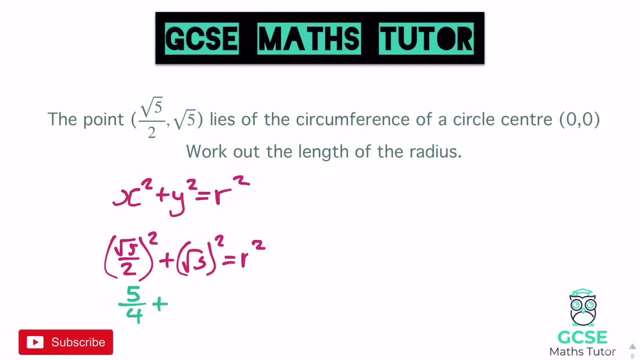 So that's 5 quarters plus Root 5 squared, or root 5 times root 5 is just the whole number 5.. There we go, And we're going to have to work that out. So 5 and a quarter plus 5.. 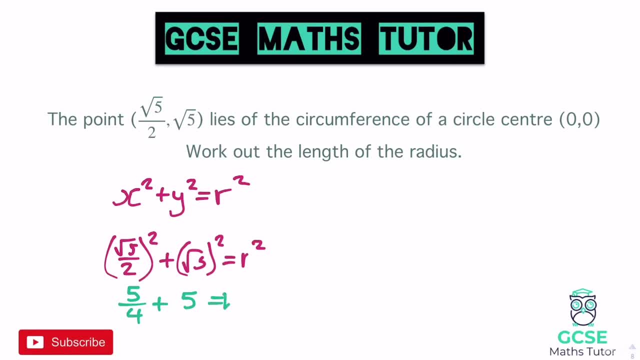 Now 5 and a quarter is 1 and a quarter, So I could rewrite this again. So I've got 1 and a quarter plus 5, which adds together to make 6 and a quarter. There we go, And that there is our radius squared. 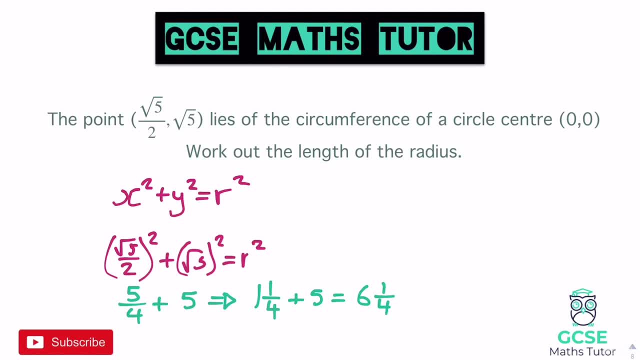 So we could actually write the equation of the circle from this. But let's have a look Now. this, without a calculator, is something we're going to have to square root that to actually find the length of the radius now, Because that is our r squared. 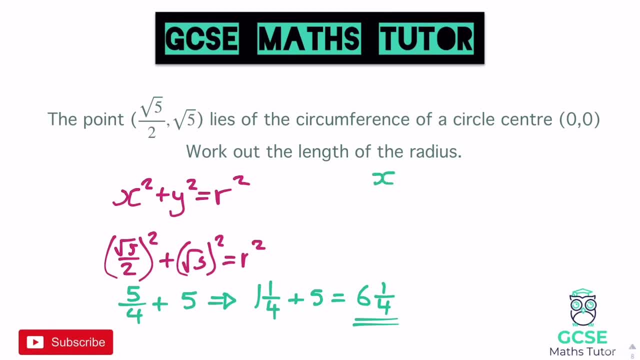 So we could actually write the equation of the circle. We could say: x squared plus y squared equals 6 and a quarter. But now we actually have to be able to square root this. So square rooting this without a calculator is a little bit trickier. 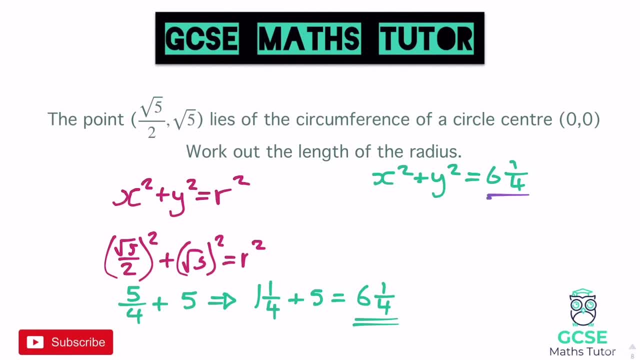 But we actually have looked at this method earlier in the video. I need to make this here a top heavy fraction. If I have a calculator, nice and easy, You just type it in. Let's have a look at doing it without a calculator. 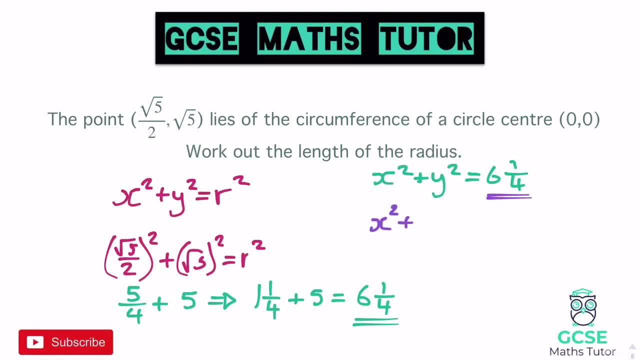 So we have x squared Plus y squared Equals, and if we make that top heavy 6 times 4 is 24.. Add the 1 is 25.. So it's 25 over 4.. Right, So to get the actual, the actual radius here. 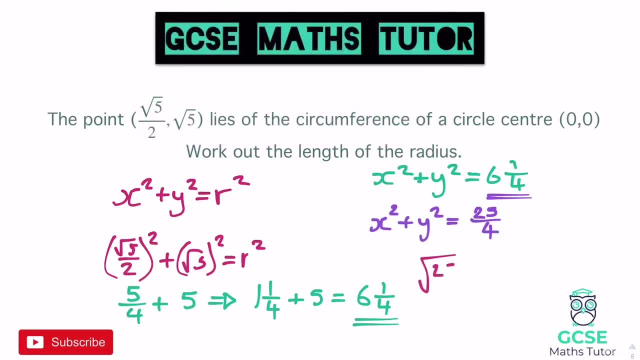 We need to square root 25 over 4.. So square root 25 over 4 and you'll notice, hopefully, that those two are nice square numbers. So the square root of 25 is 5.. Square root of 4 is 2.. 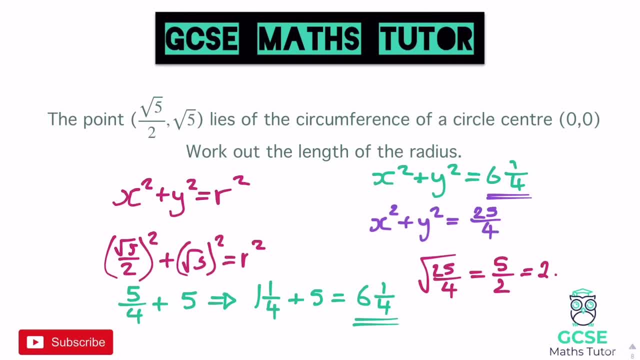 So it's 5 over 2., Which you could write as a decimal as well. You could write that as 2.5. And again, if you just typed it straight into a calculator, it probably would have given you 2.5 straight off. 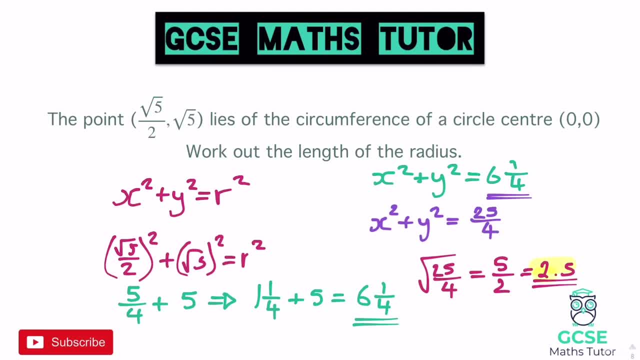 But there we go. There's the length of the radius 2.5.. Right, Quite a lot of steps there. Probably could have skipped some of the steps that I'm writing down. I don't really need to write out the equation of the circle every time and rewriting it. 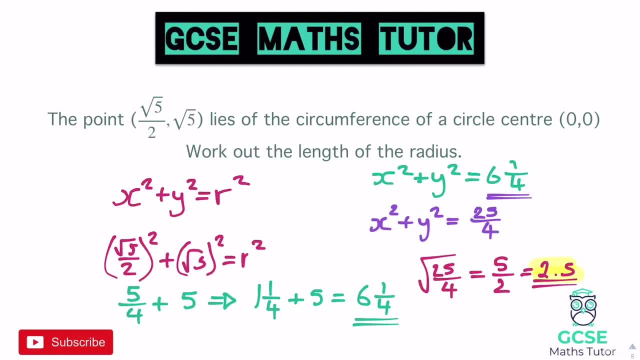 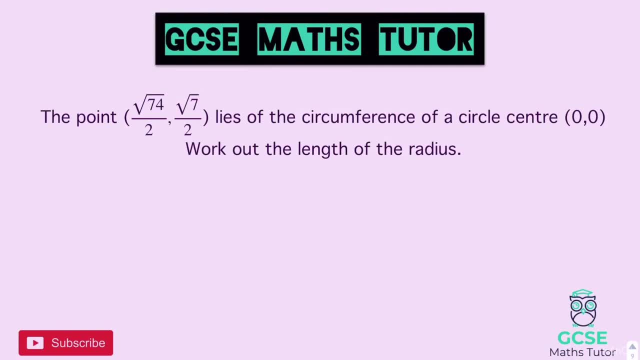 But it's quite a good practice just to get into writing it out straight away So that you recognize that equation Right. Here's the last question for you to have a go at then. Okay, So this is very similar to the one. 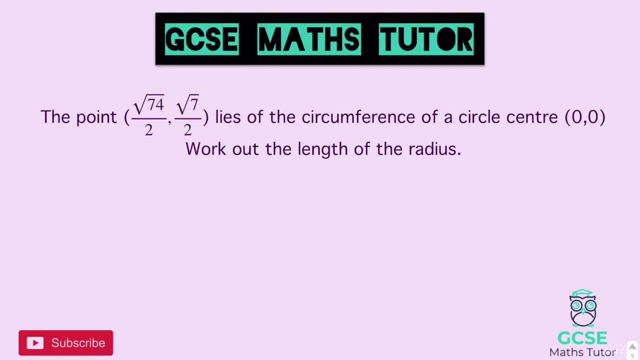 I've just done. You've got two third coordinates there, So sub that into the equation of the circle and try and find the length of the radius. So pause the video there. We'll go down to in a sec, Right, Okay? 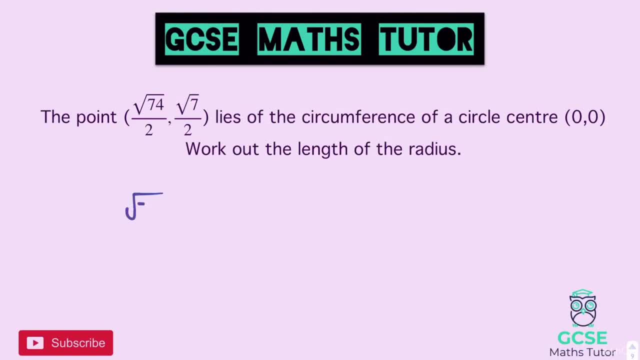 So let's plug these in. So we have root 74 over 2 squared is our x squared, Plus root 7 over 2 squared is our y squared, And that's going to equal the radius squared. Okay, So Squaring the left one there.